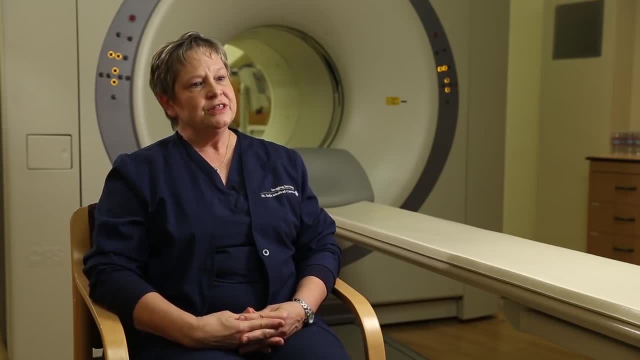 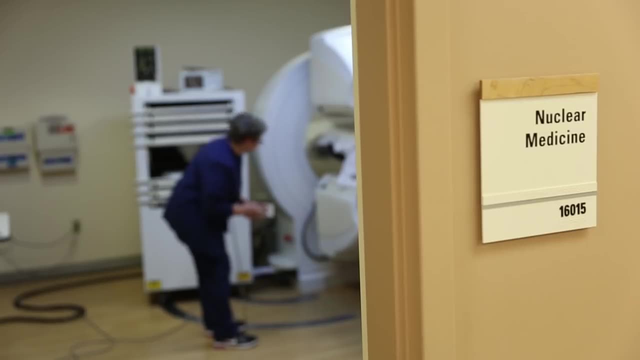 the situation. Communication is very important. You need to be able to talk to all different kinds of people: doctors, patients. You need to have some computer background, of course, a good science background, anatomy, physiology background. Sometimes, believe it or not, 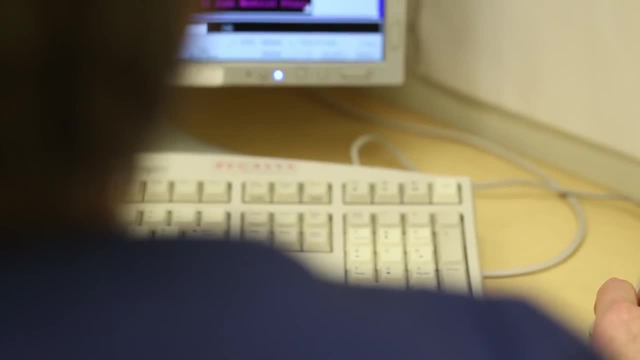 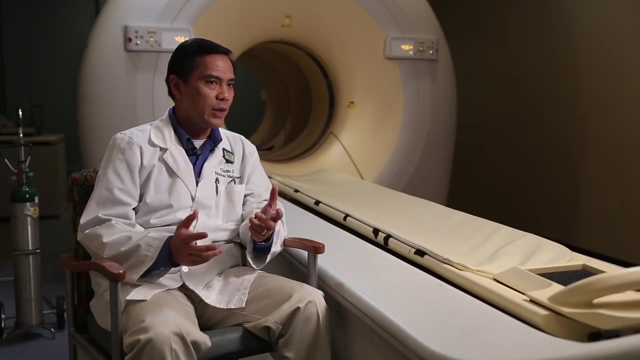 organs are not in the exact same spot in every patient, so you have to try to figure out. hmm, is that what I'm looking for, or is it not? What makes my profession different is that we get to play with a lot of technologies. 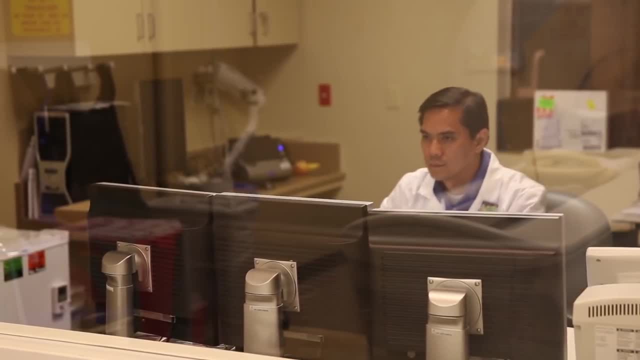 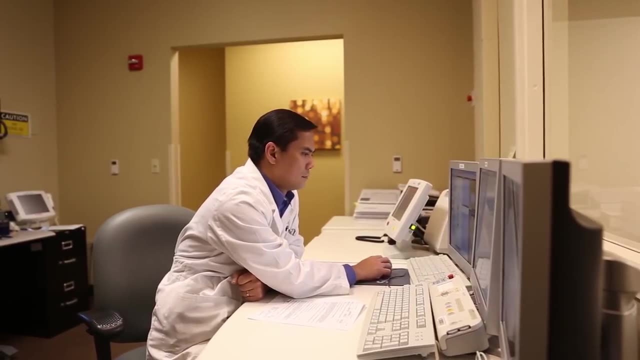 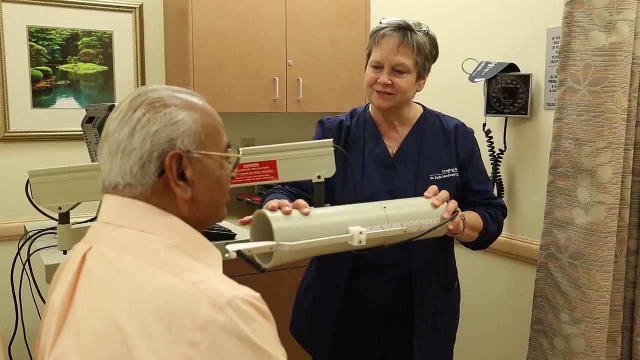 Right now we're in the forefront of fusion imaging, which is combining CT with nuclear medicine, MRI with nuclear medicine. Well, I've always enjoyed what I do and I think it probably is more because of the closeness that you can have with your patients. You have a real rapport with the doctors. that 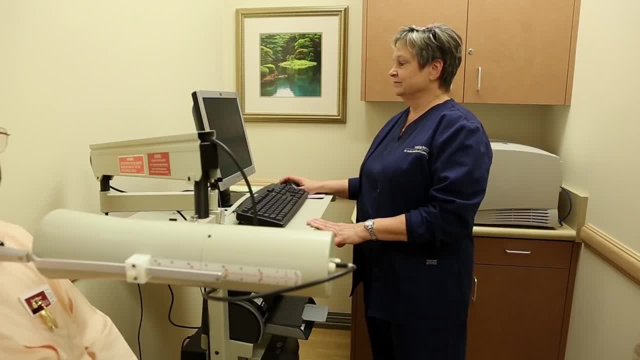 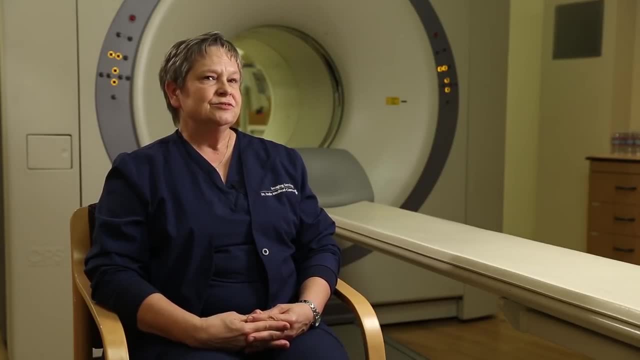 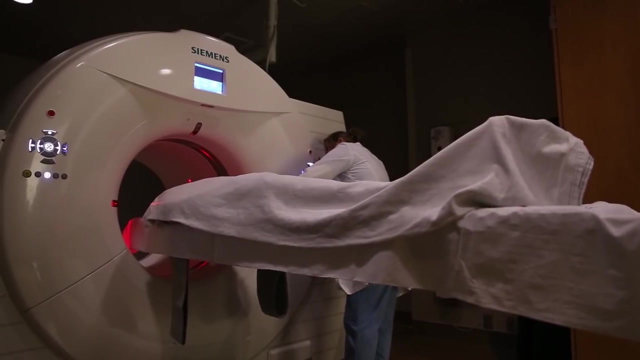 you work with also And again you work with cardiologists and oncologists and radiologists, so you work with a real gamut of people and you do so much good for the patients. We did a WBC scan, That's a white blood cell scan. We tagged the blood cells of the patient. 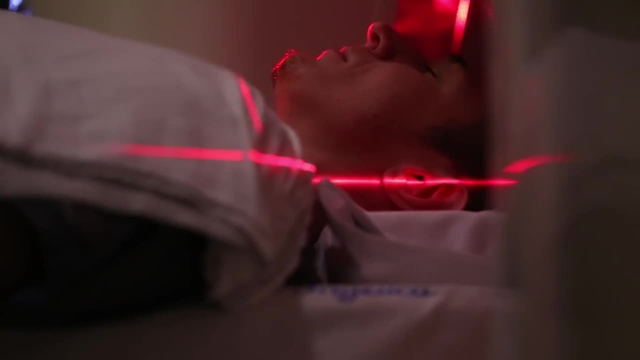 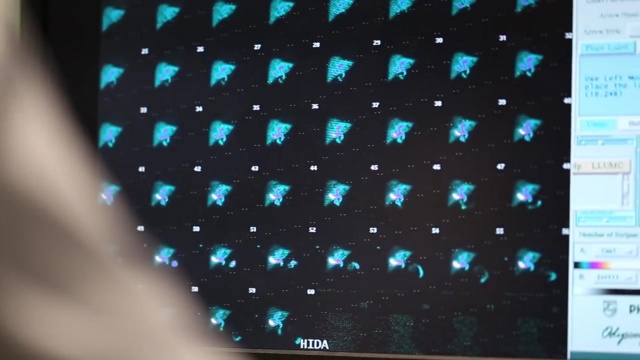 and we re-inject them so we're able to see where that tracer goes. They did not know what was wrong with this patient. This patient had a fever and couldn't figure out what was wrong, and this was able to identify infection that they were. 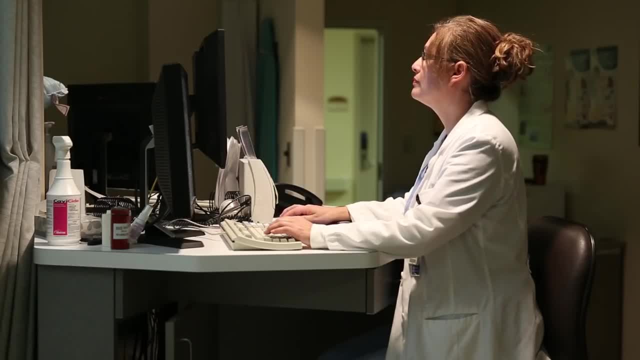 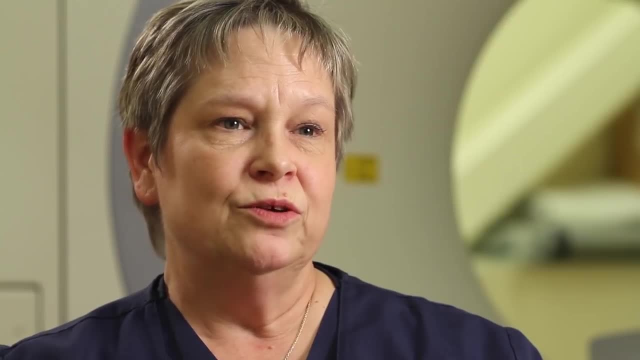 unable to see with other diagnostics. I mean, really it could have saved the patient's life and that really made me feel good and we really took part and helped save that patient. I think because we deal with so many oncology patients, cancer patients, you can see them. 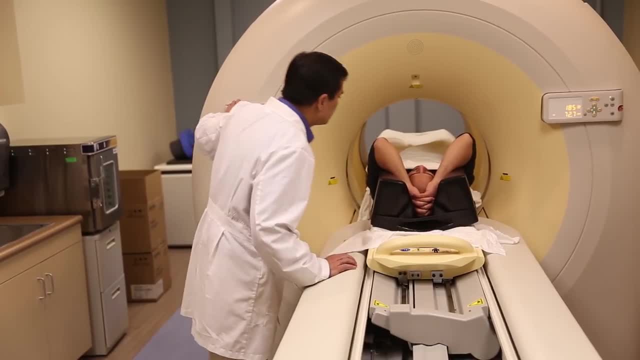 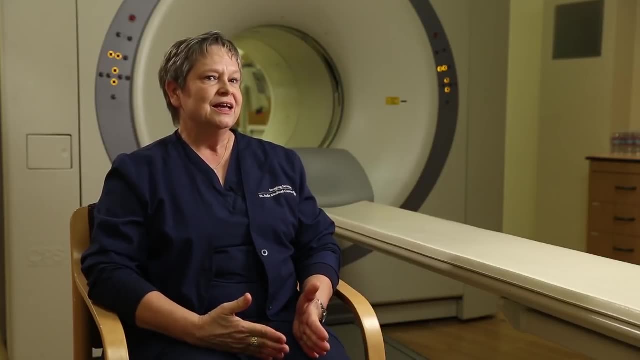 through different stages of their initial diagnosis- You see them as they're going through their treatments- and to be able to see a person who you knew was very ill and to see them walking around and living their life and living a good life. I think it's really important to be able to see a person who you knew was very ill and to see them walking around and living their life and living a good life. 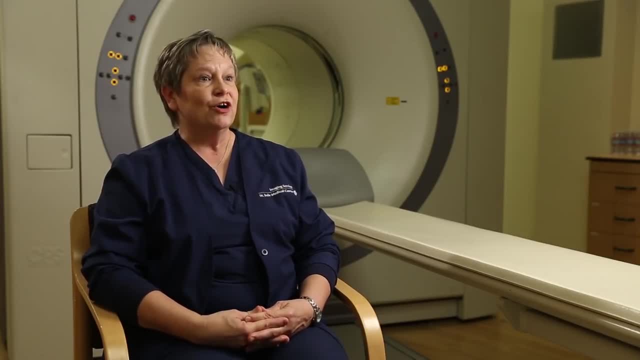 I think it's really important to be able to see a person who you knew was very ill and to see them walking around and living a good life After their treatment. you really feel a part of that. Well, for people that are interested in technology and science, I think it would be really very. 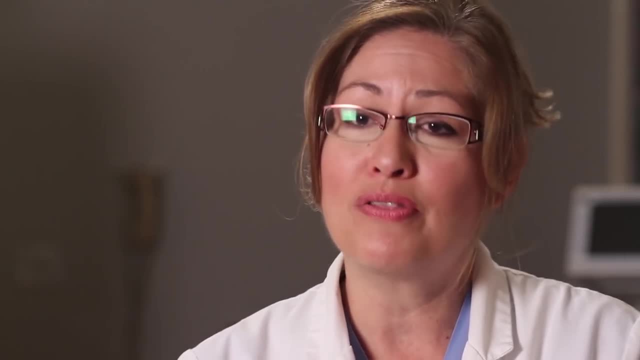 interesting for them. It pays well too, so you have all the benefits. really, It's a great field to be in.